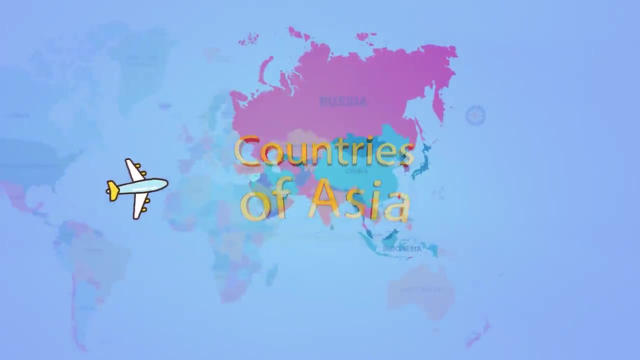 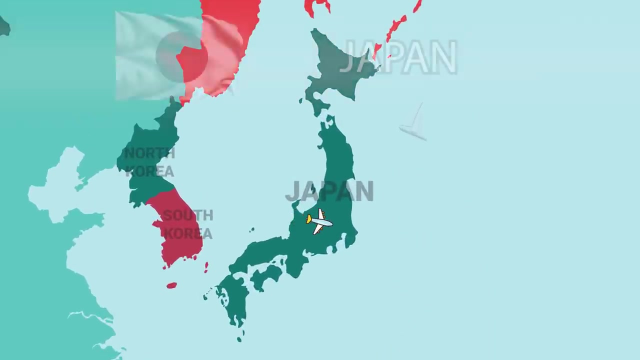 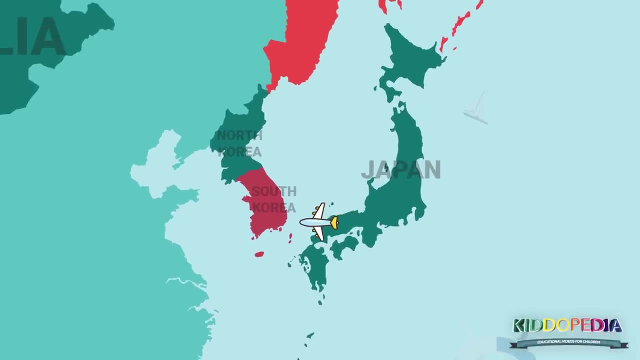 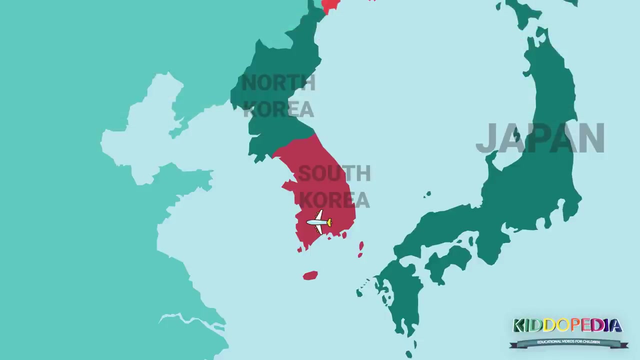 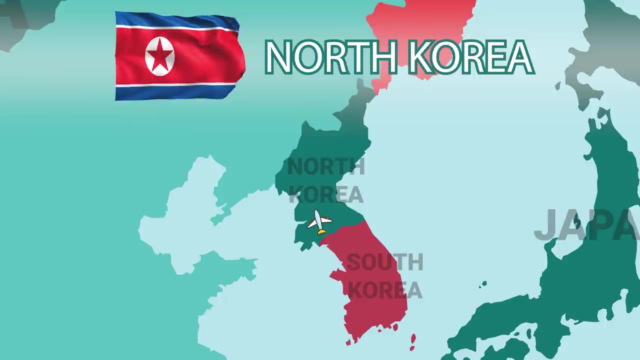 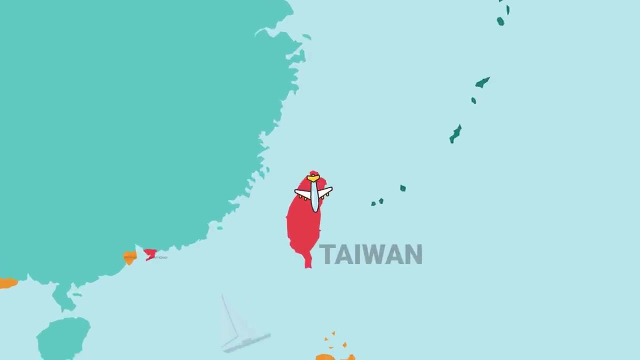 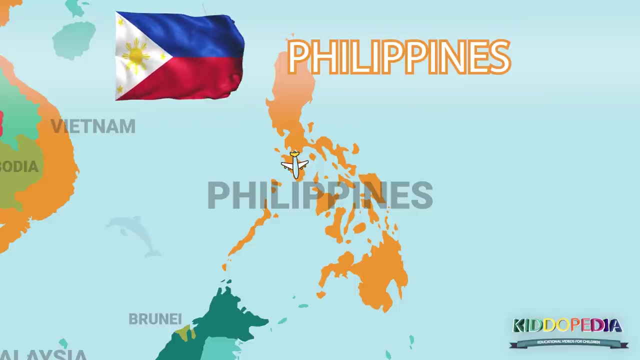 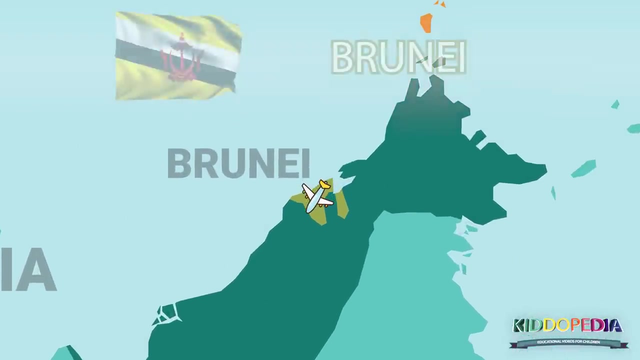 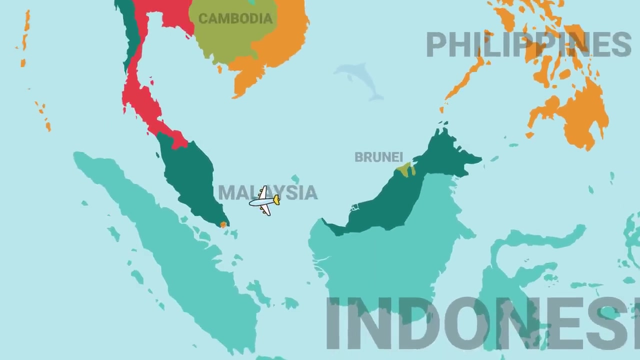 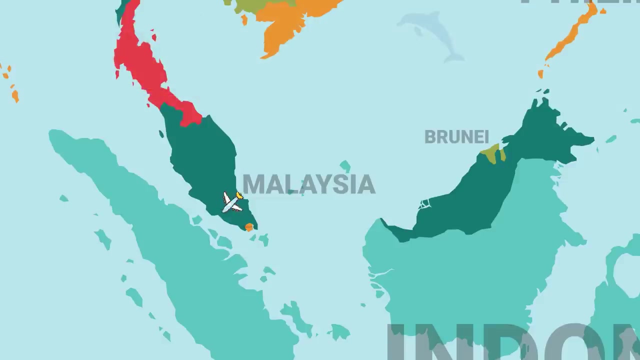 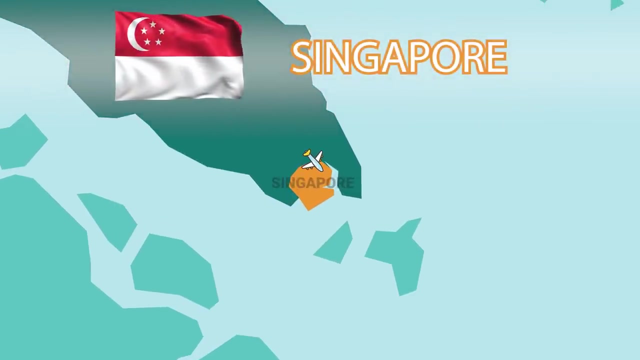 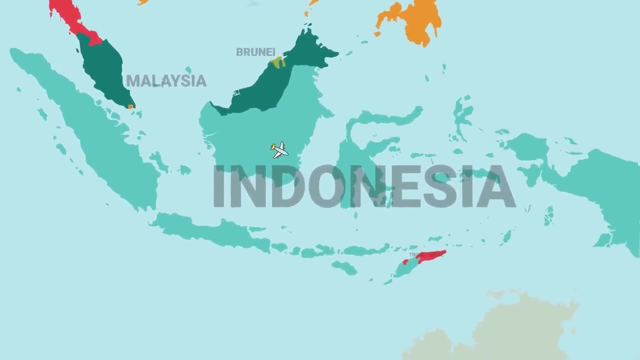 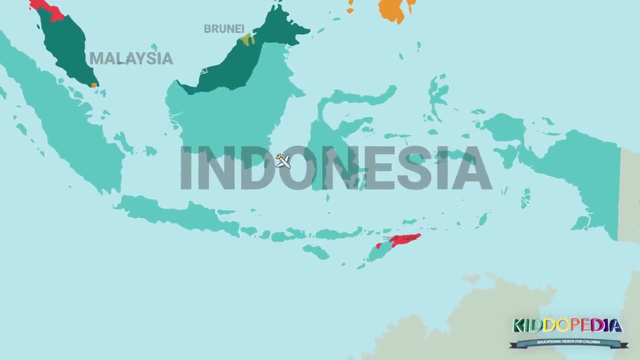 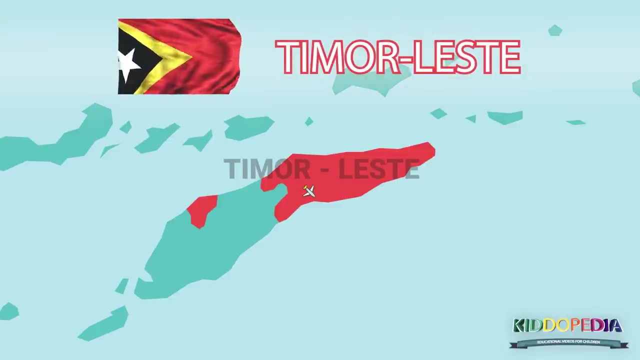 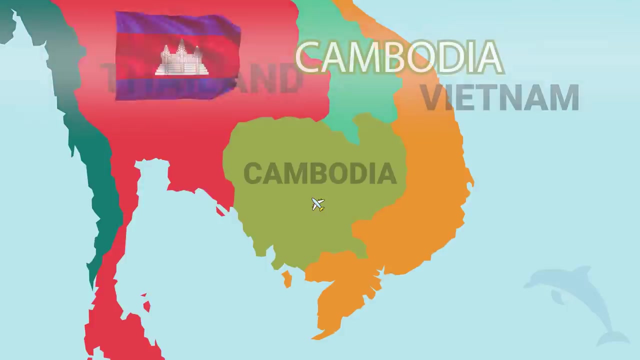 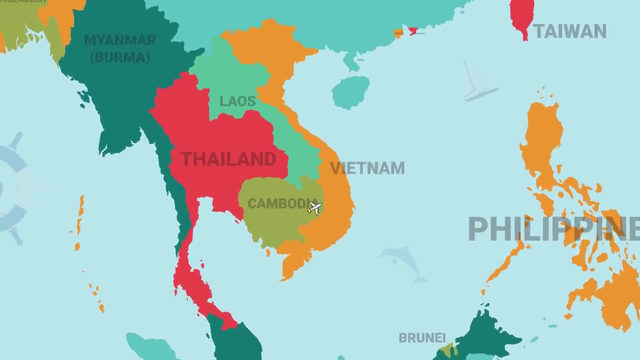 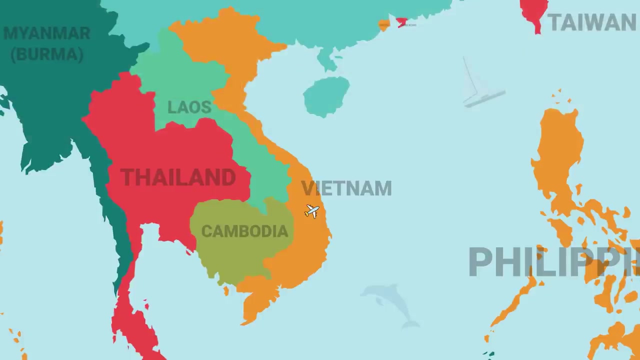 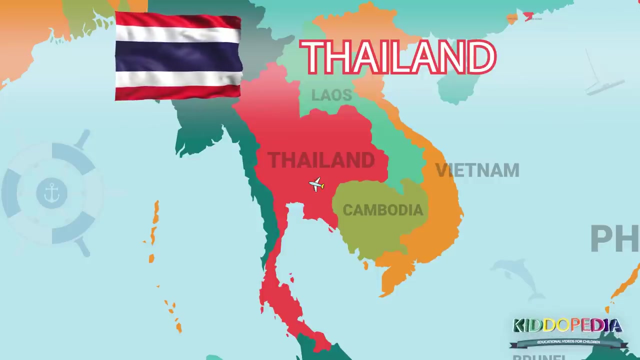 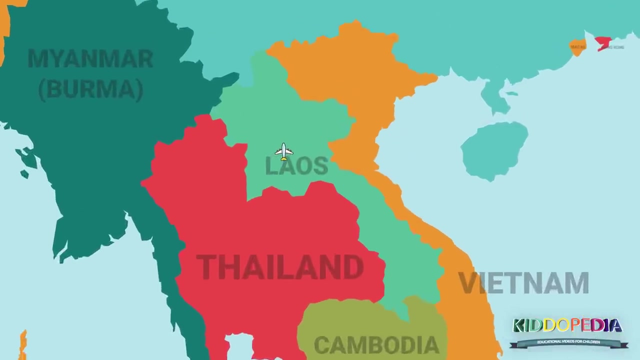 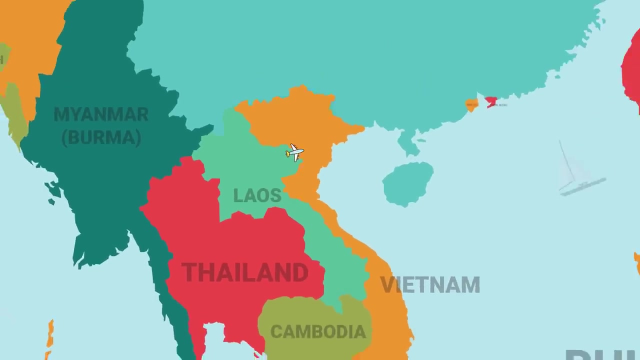 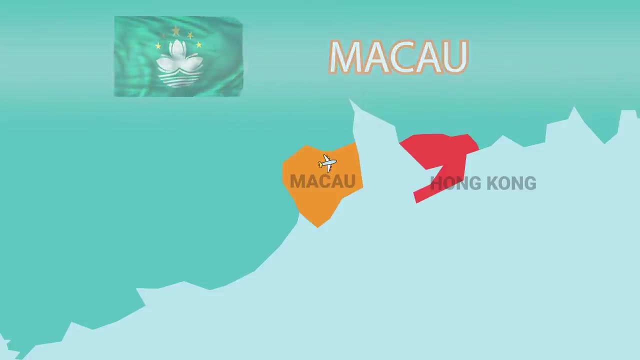 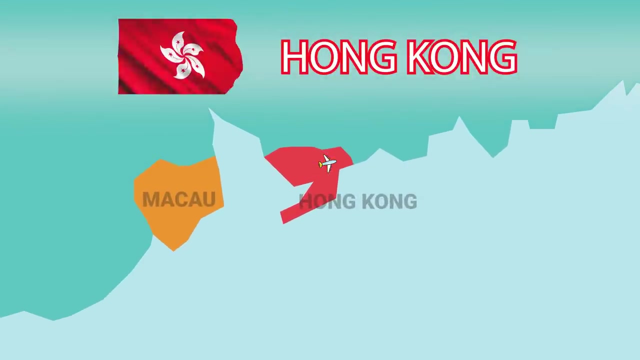 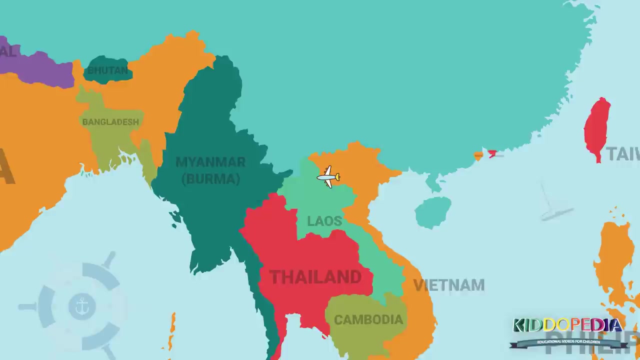 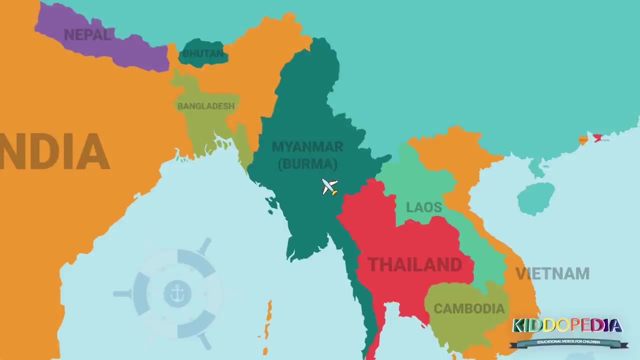 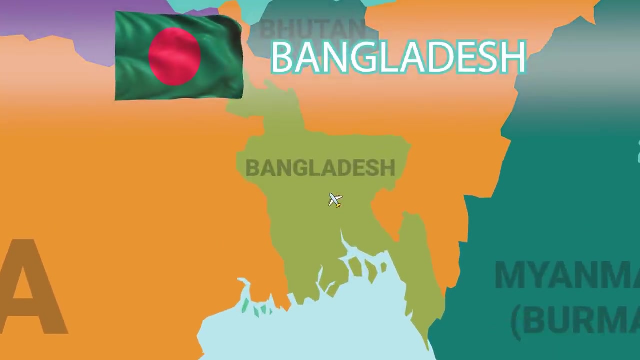 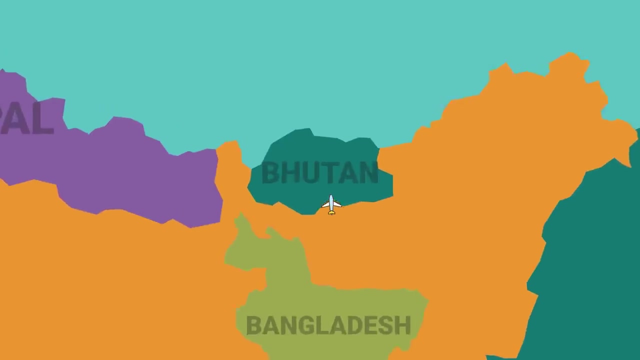 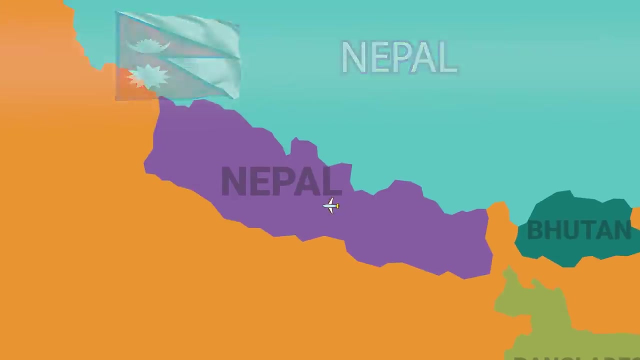 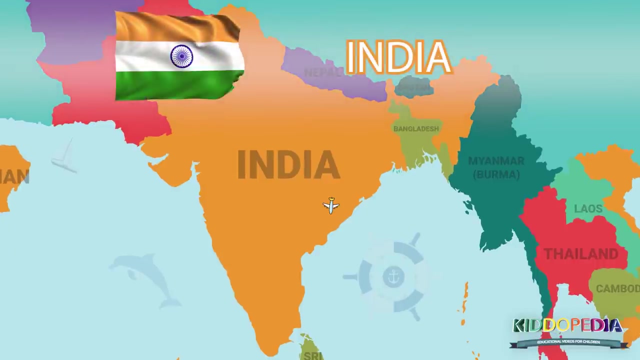 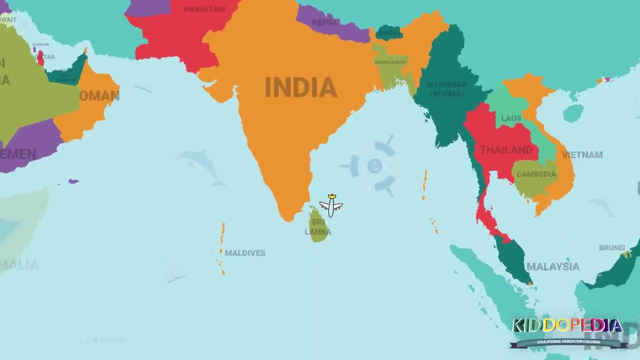 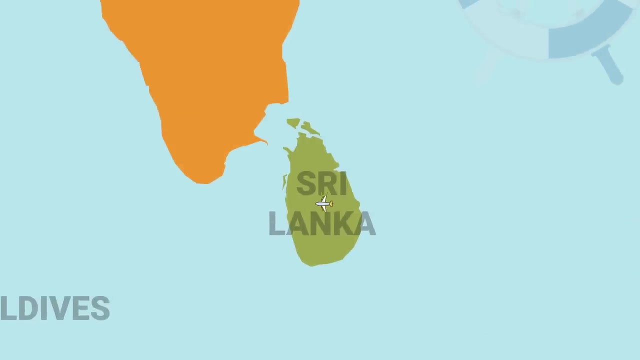 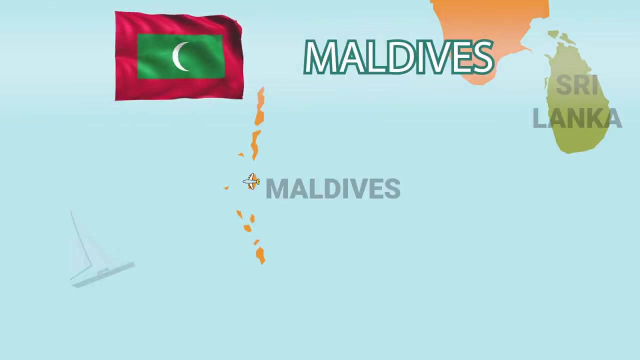 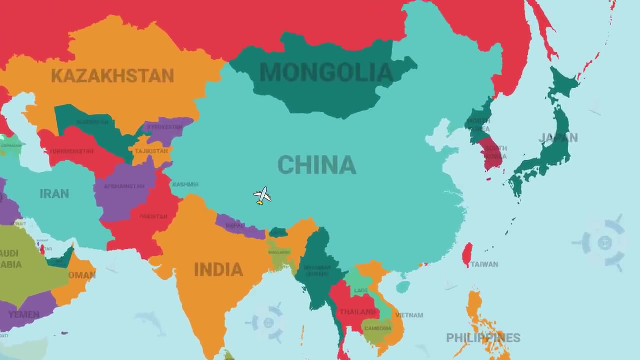 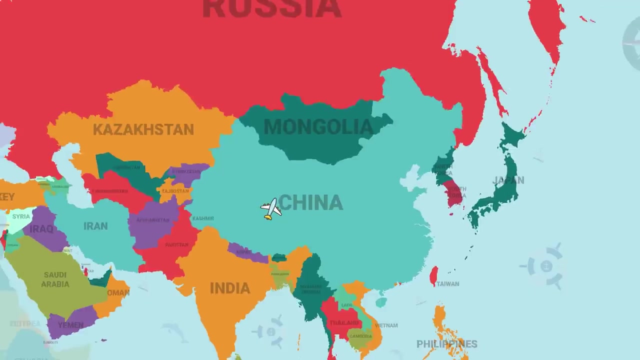 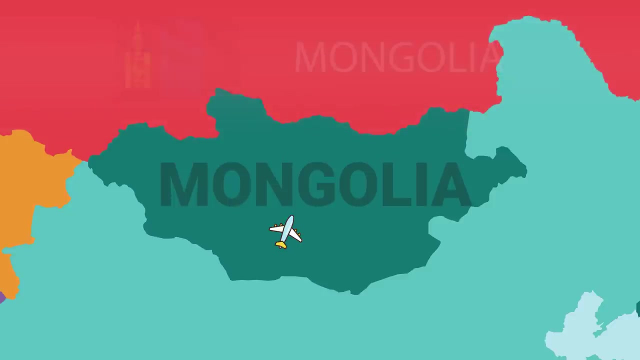 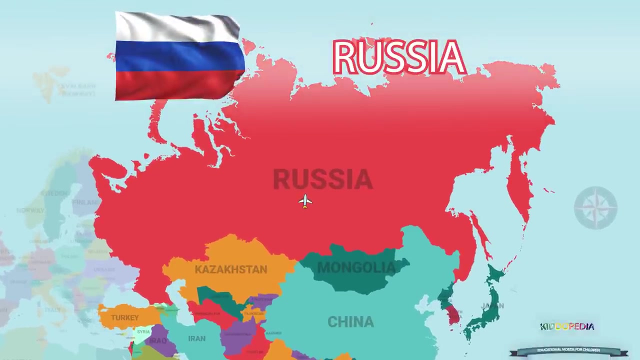 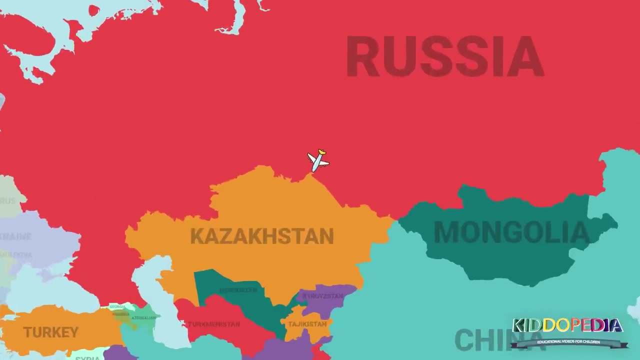 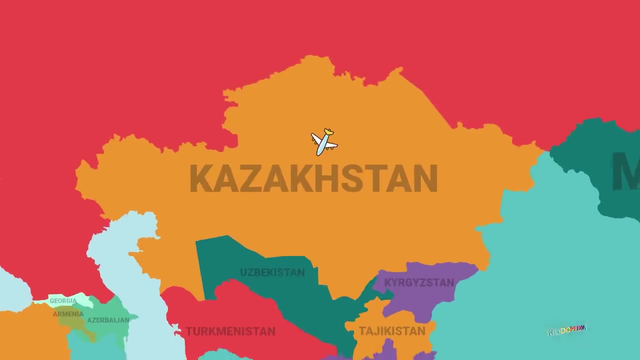 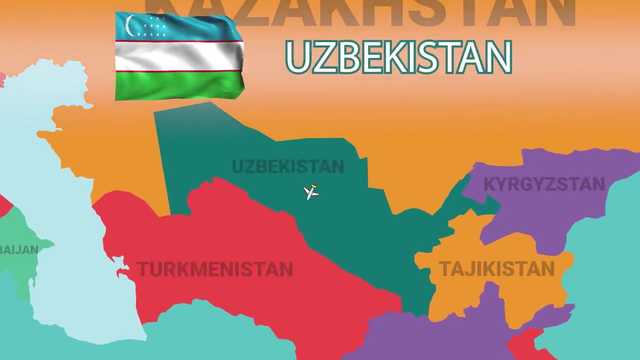 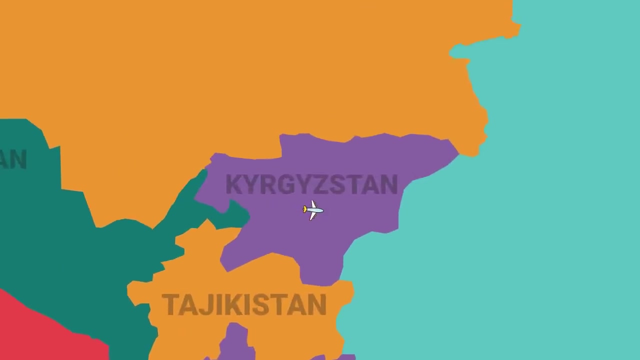 Countries of Asia: Japan, South Korea, North Korea, Taiwan, Philippines, Brunei, Malaysia, Singapore, Indonesia, Timor Leste, Cambodia, Vietnam, Thailand, Laos, Canada, Macau, Hong Kong, Myanmar, Bangladesh, Bangladesh, Bhutan, Nepal, India, India, Bangladesh, UP, Maldives, China, Mongolia, Russia, Kazakhstan, Uzbekistan, Kyrgyzstan, Tajikistan. 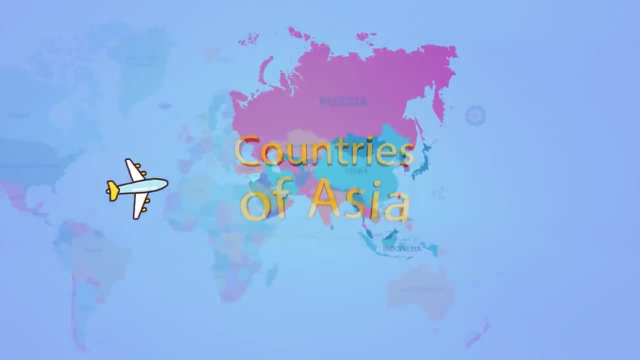 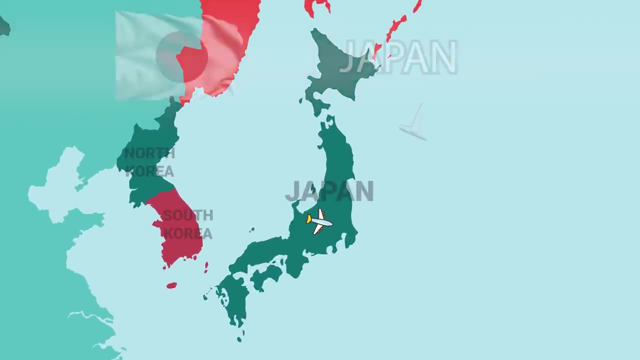 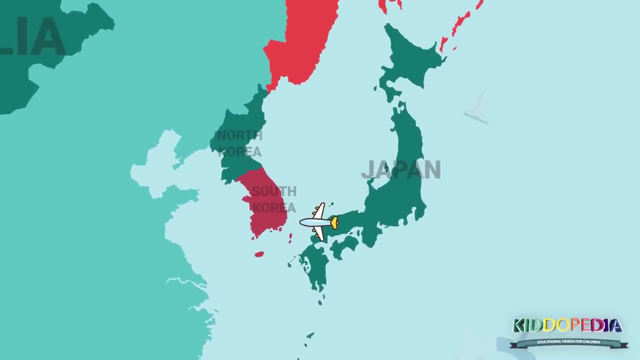 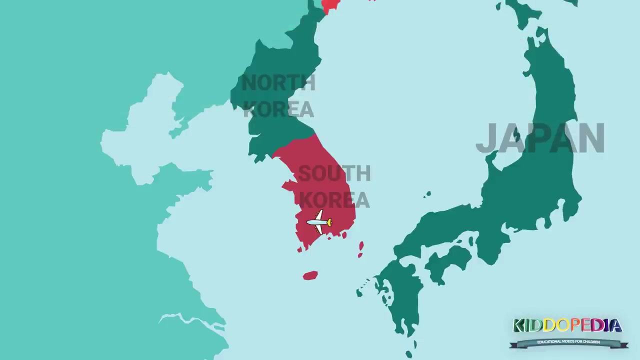 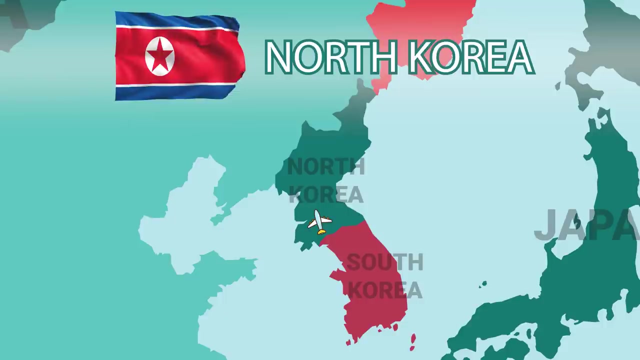 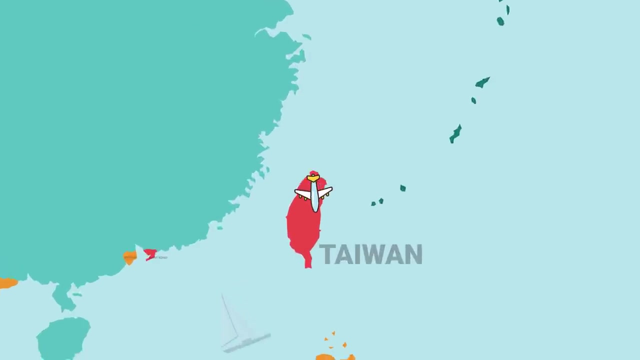 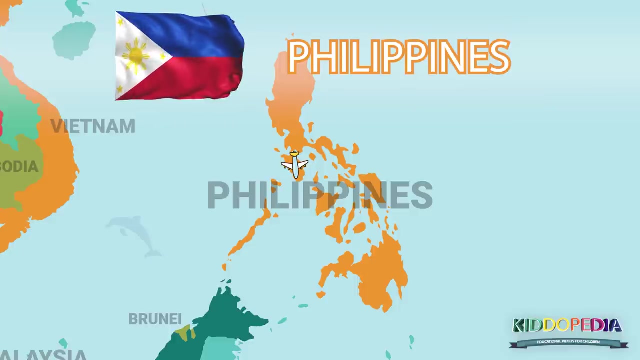 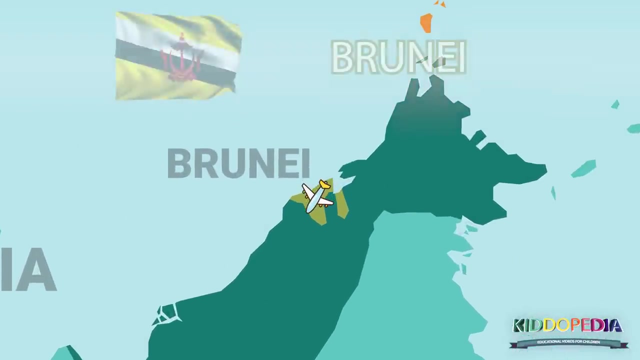 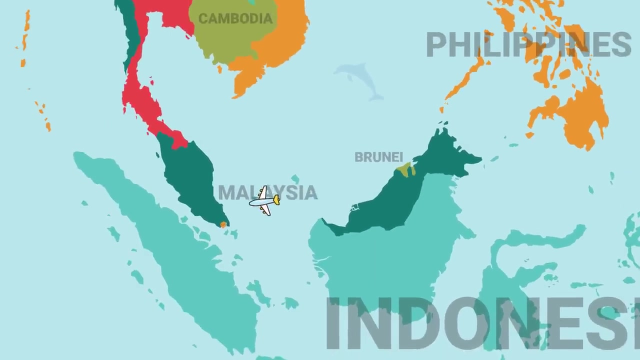 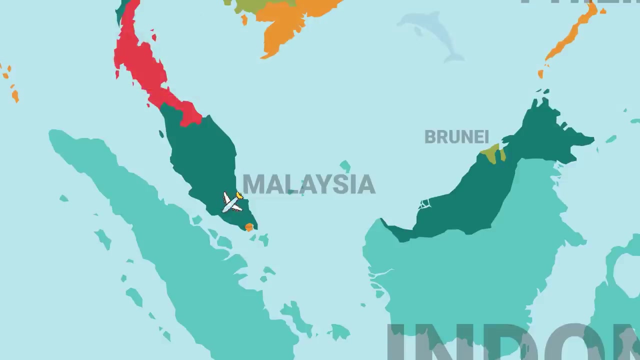 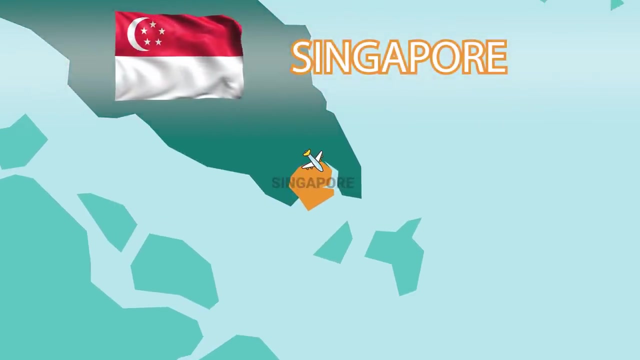 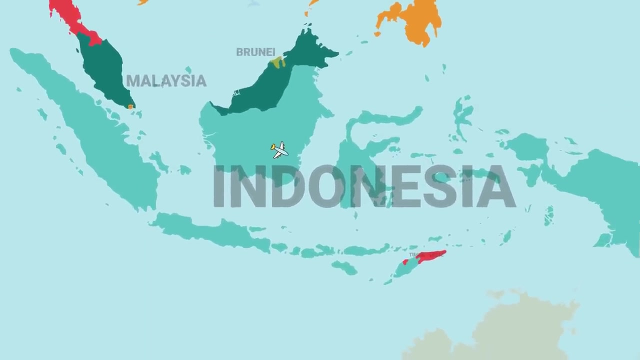 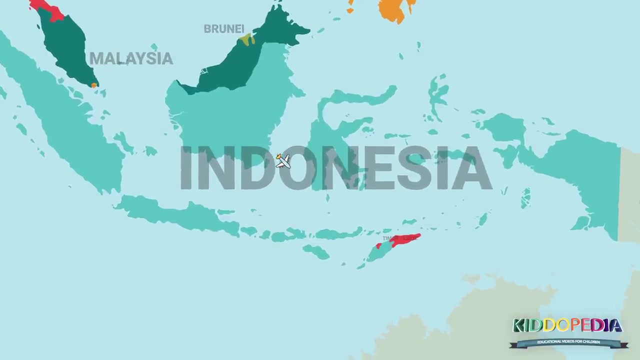 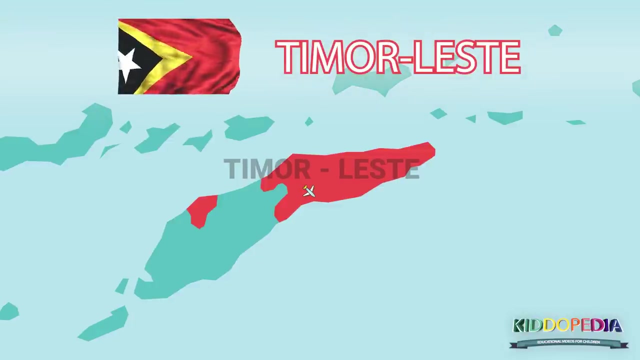 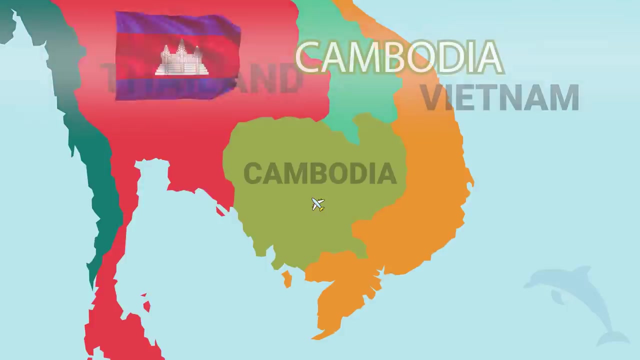 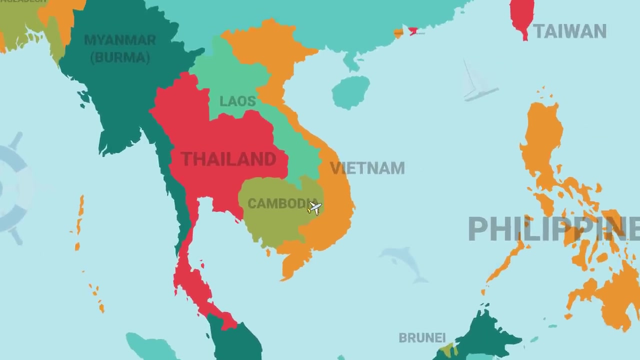 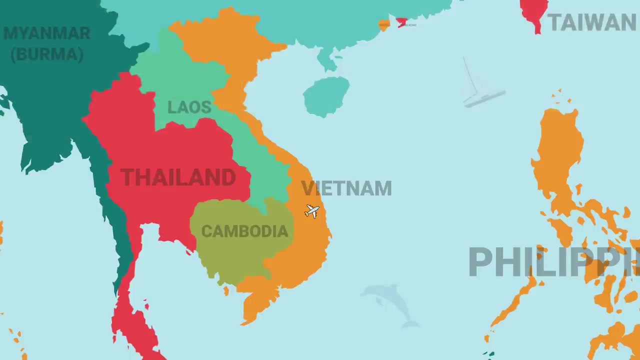 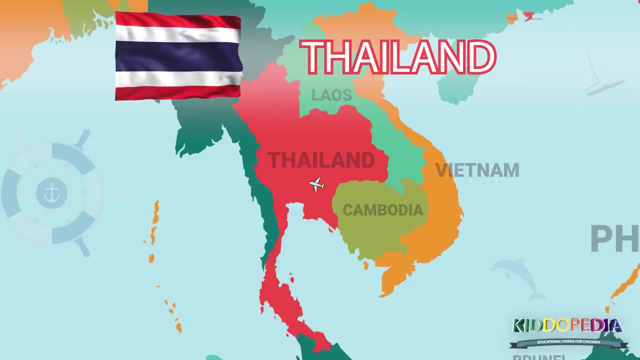 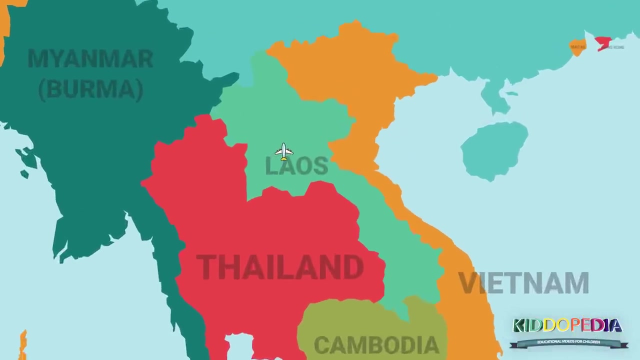 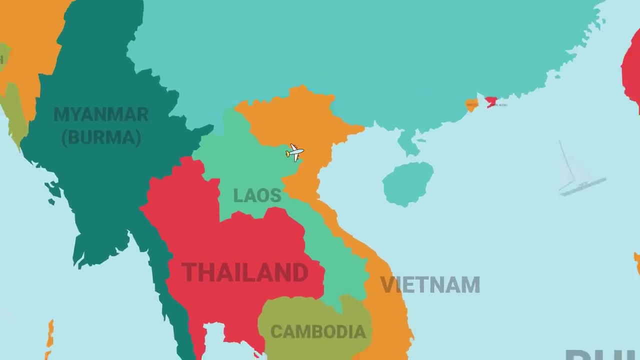 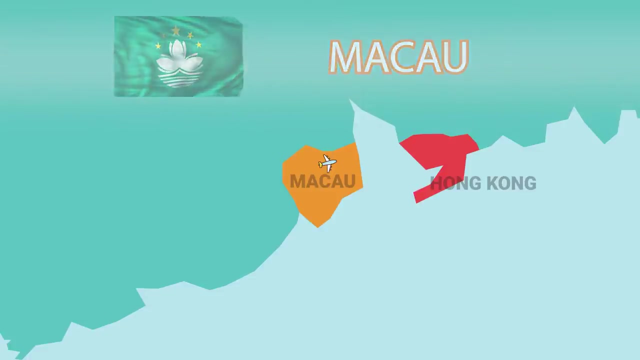 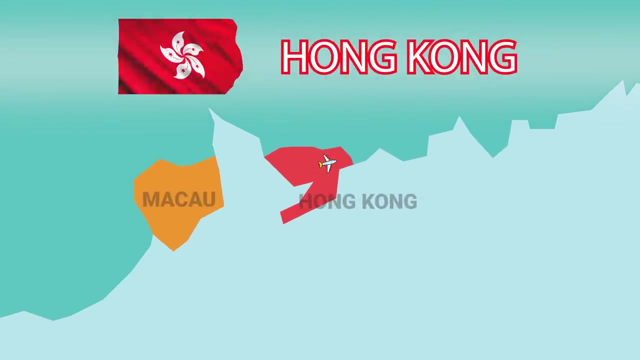 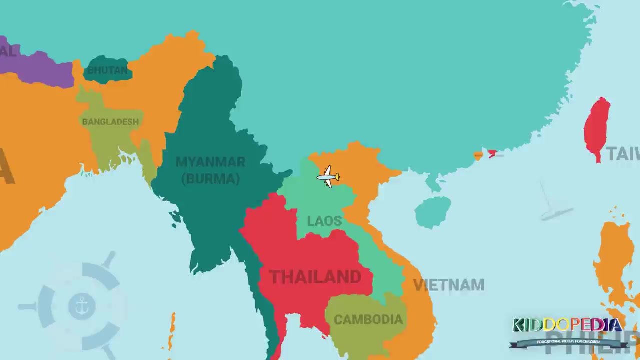 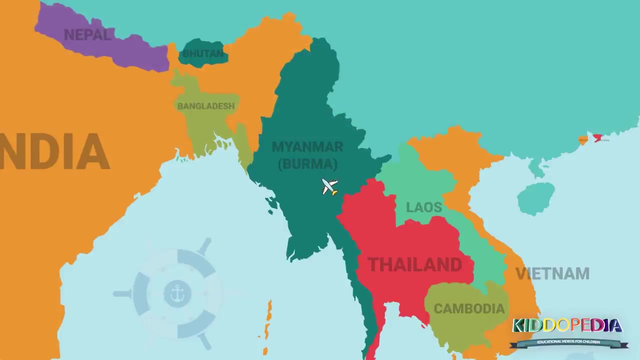 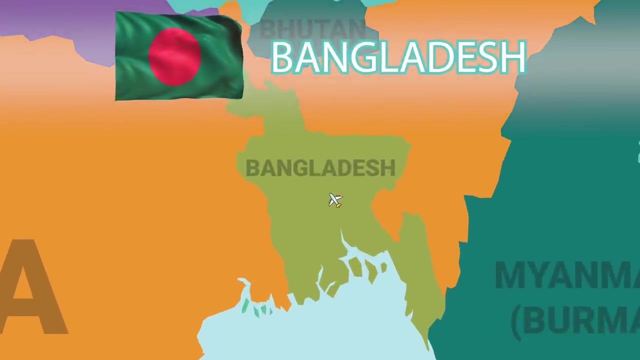 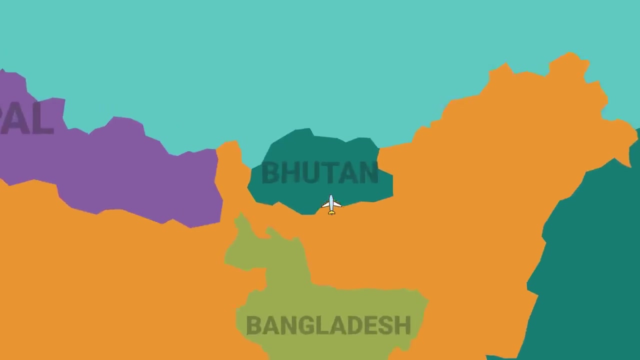 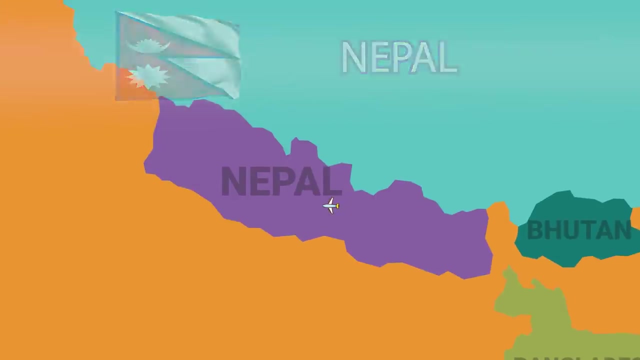 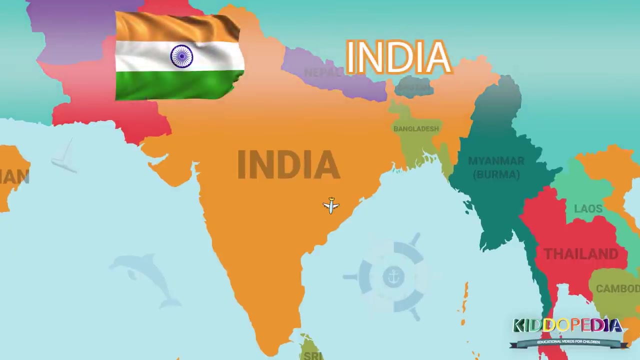 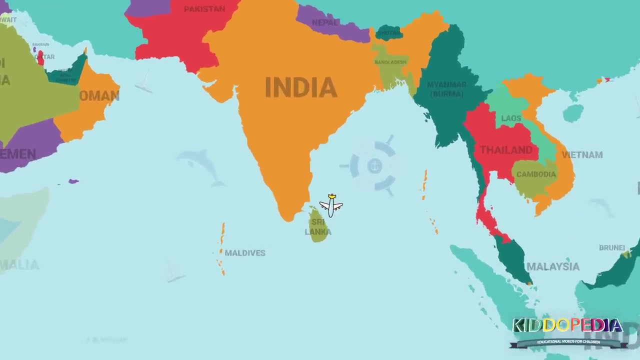 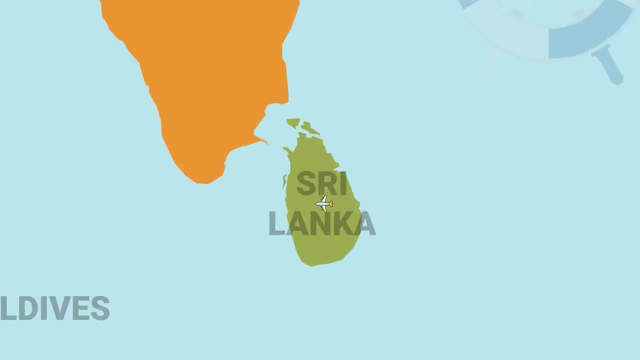 Countries of Asia: Japan, South Korea, North Korea, Taiwan, Philippines, Brunei, Malaysia, Singapore, Indonesia, Timor Leste, Cambodia, Vietnam, Thailand, Laos, Canada, Macau, Hong Kong, Myanmar, Bangladesh, Bangladesh, Bhutan, Nepal, Singapore, India, Thailand, India, Kerala, Kerala, Sri Lanka, Sri Lankan. Sri Lanka, Sri Lanka- Sri Lankan. 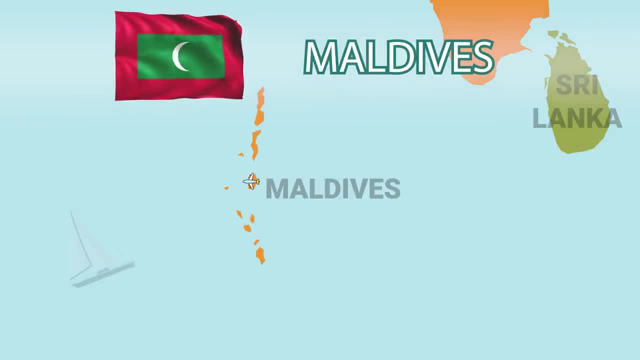 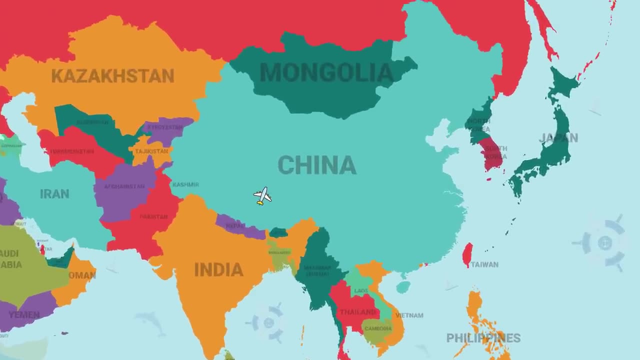 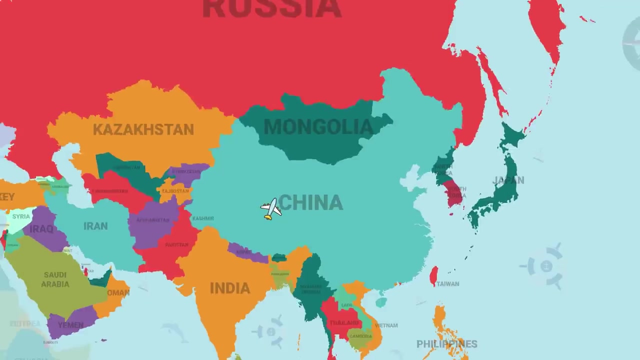 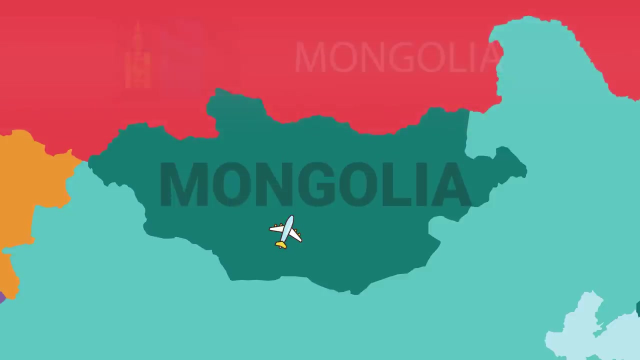 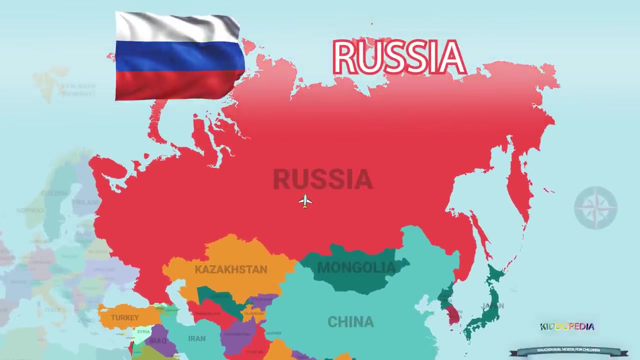 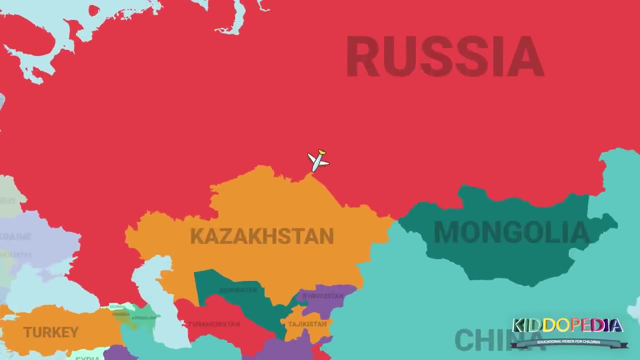 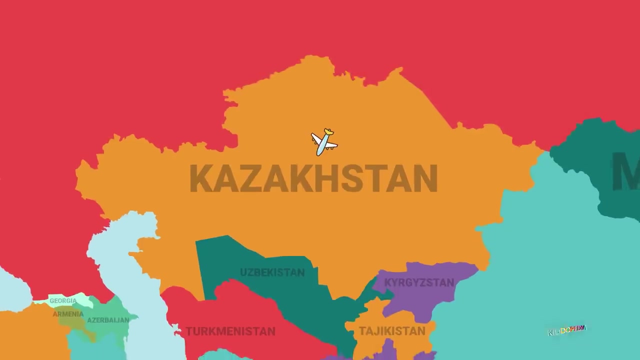 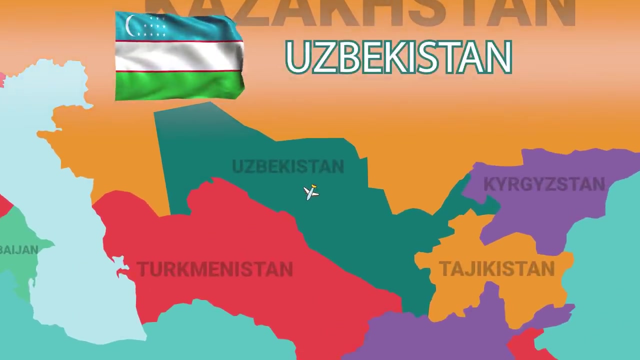 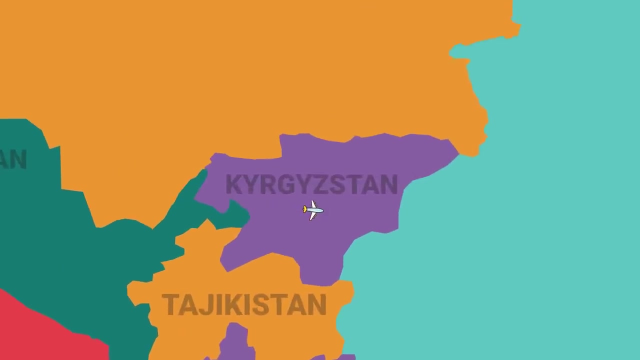 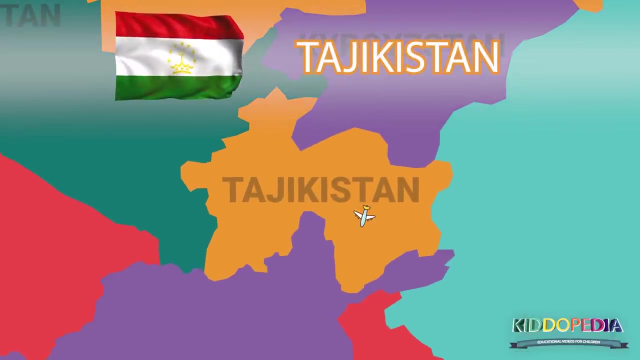 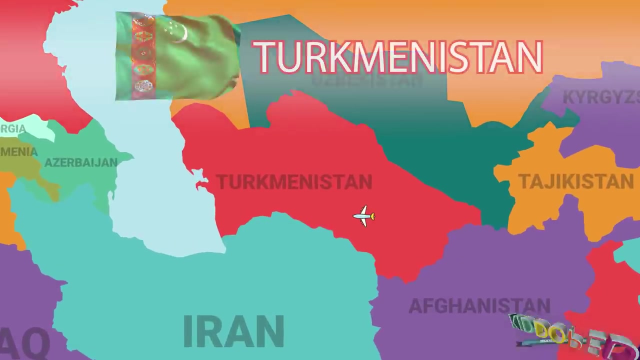 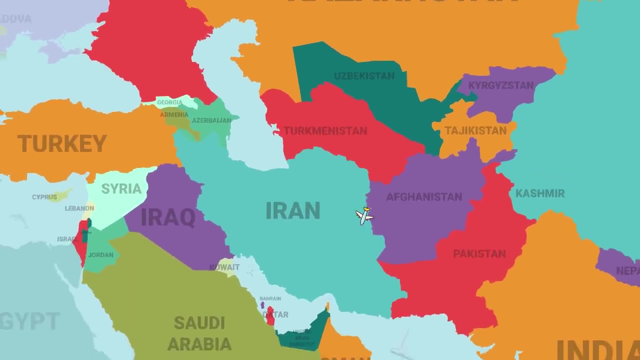 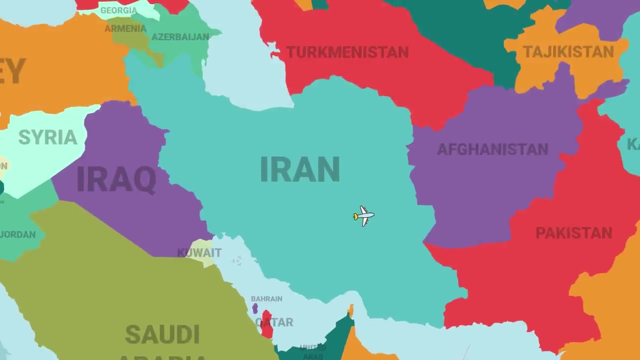 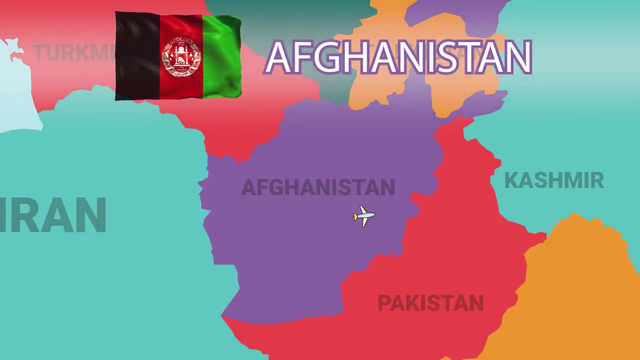 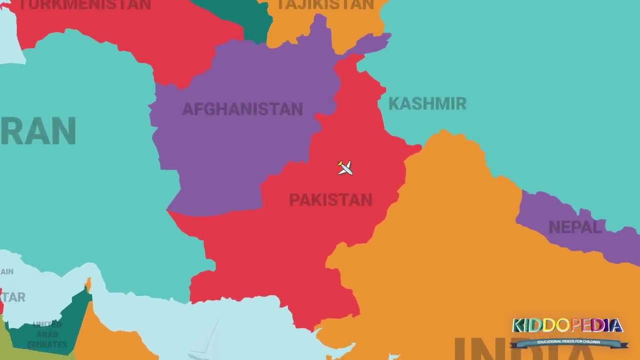 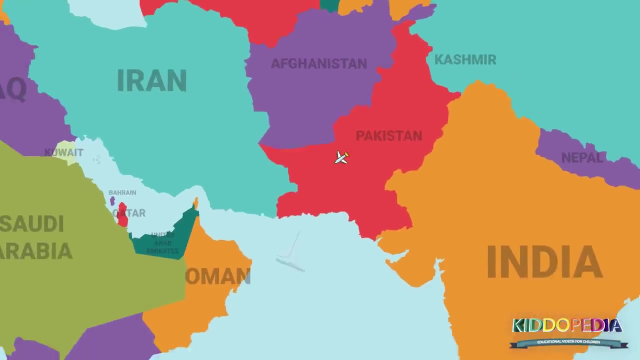 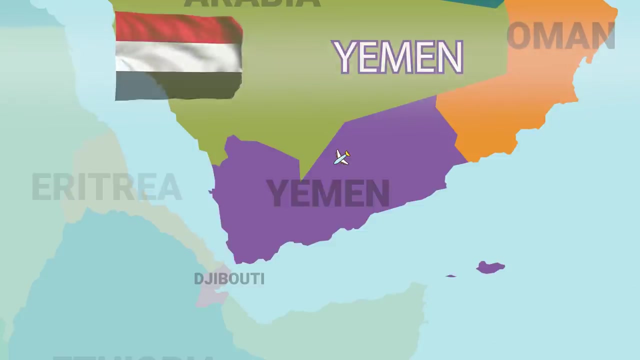 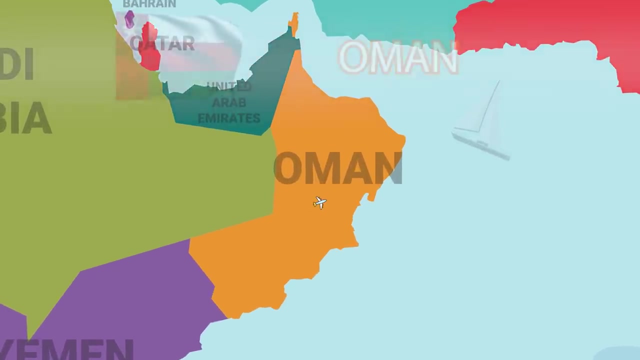 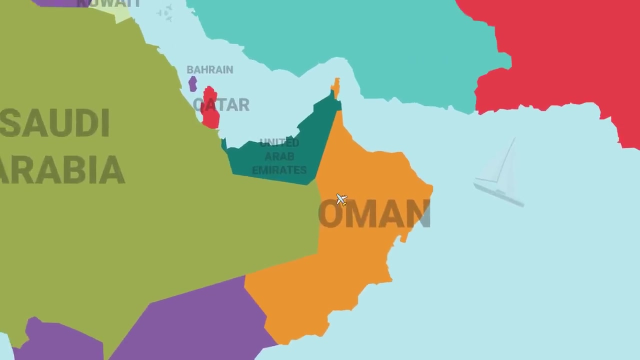 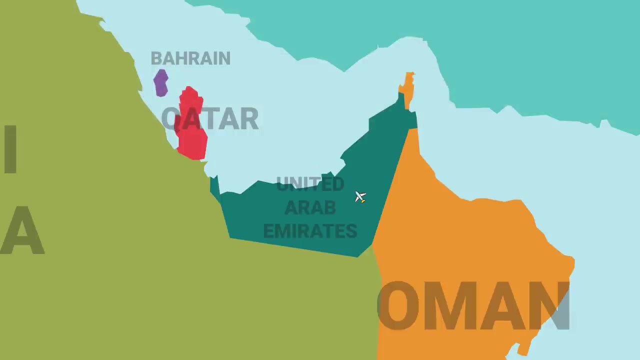 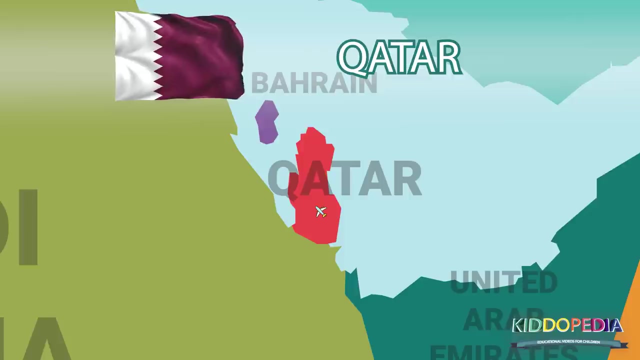 Sri Lankan. Sri Lankan Maldives. Maldives. China, Mongolia, Russia, Kazakhstan, Uzbekistan, Kyrgyzstan, Tajikistan, Turkmenistan, Turkey, Iran, Iran, Afghanistan, Pakistan, Pakistan, Pakistan, Iraq, Yemen, Yemen, Yemen. Yemen Yemen Yemen. Oman. Oman. Oman Oman Oman. United Arab Emirates. United Arab Emirates- Qatar. 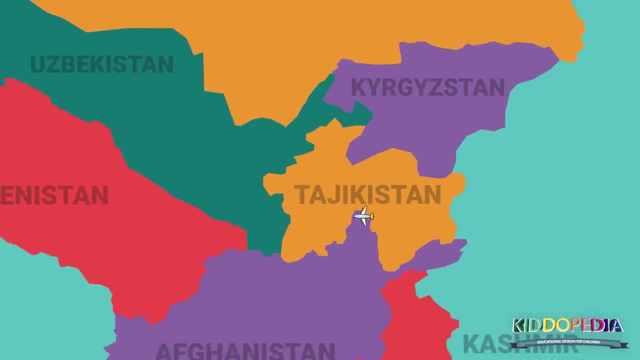 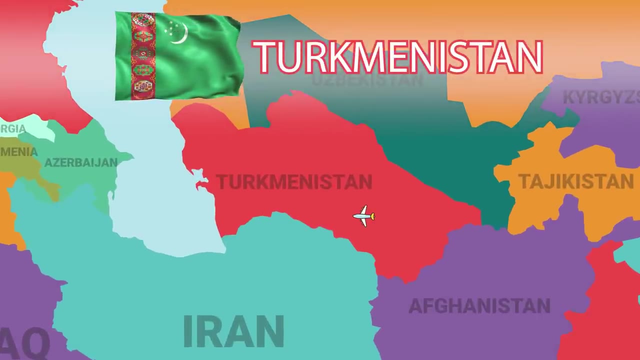 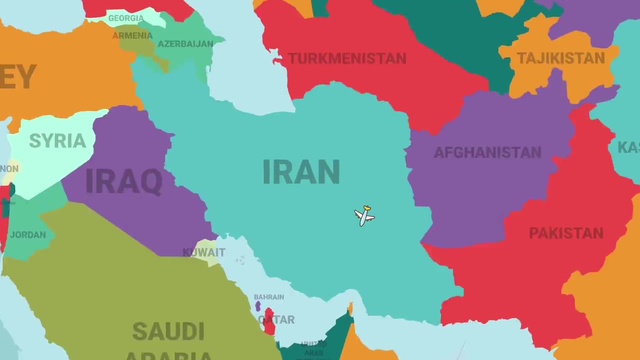 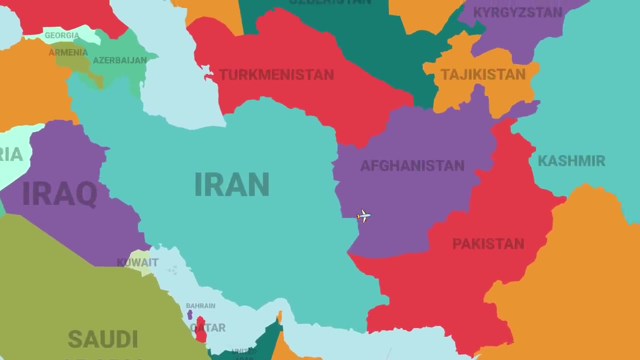 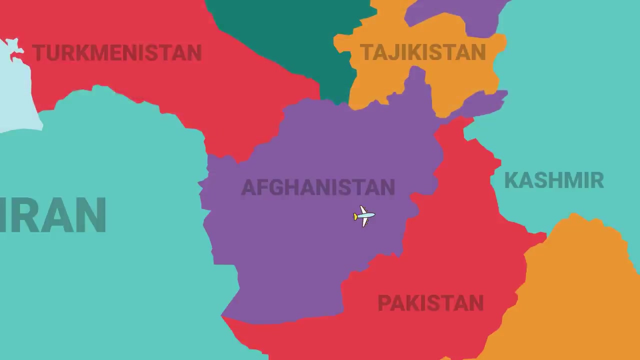 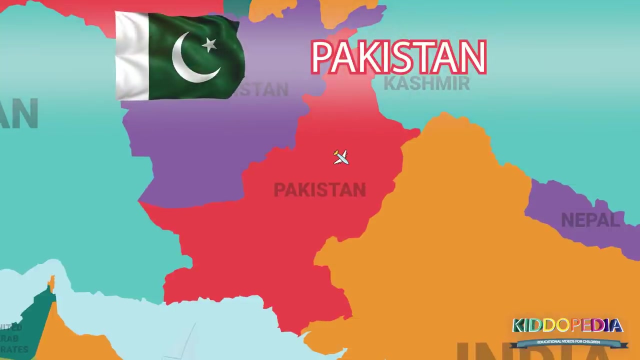 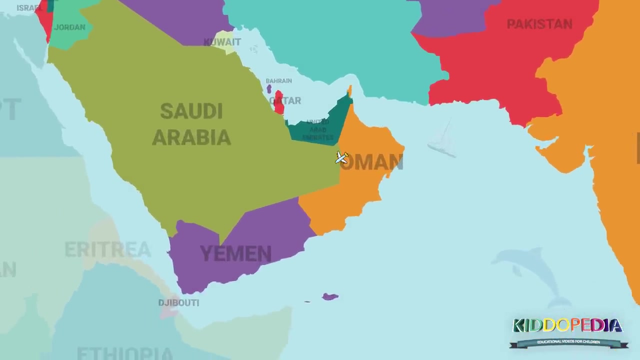 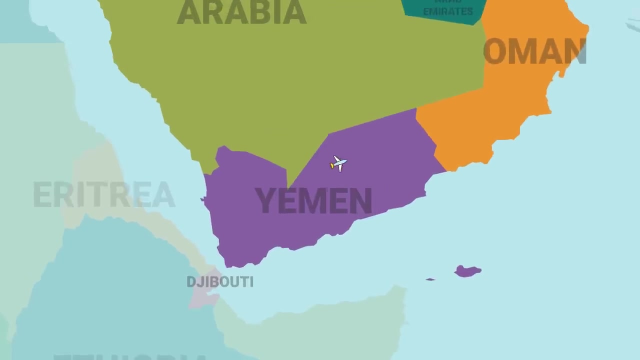 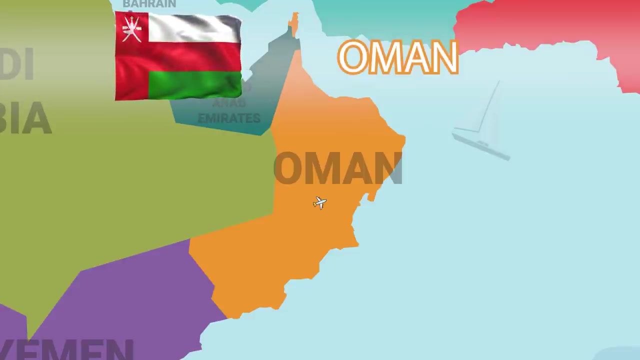 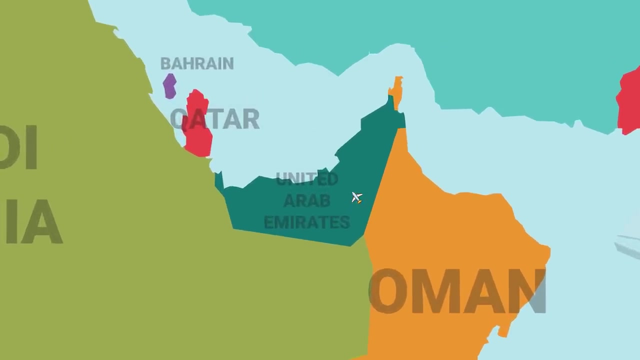 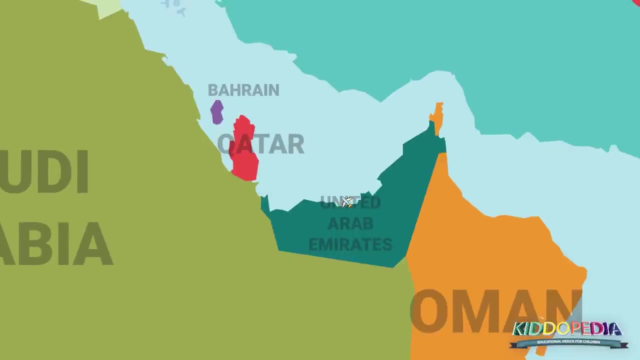 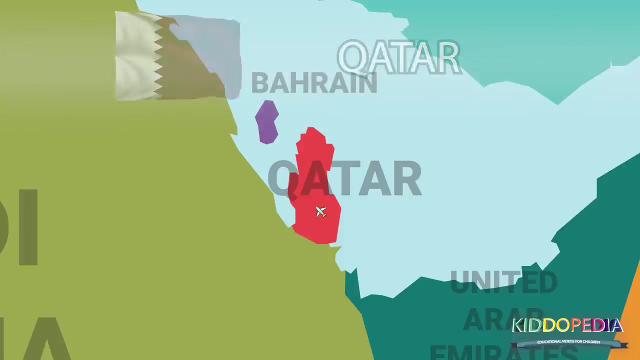 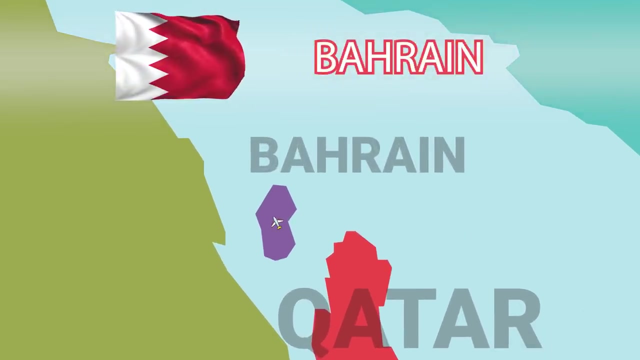 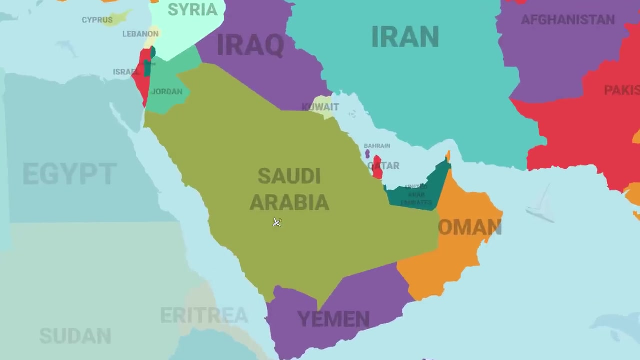 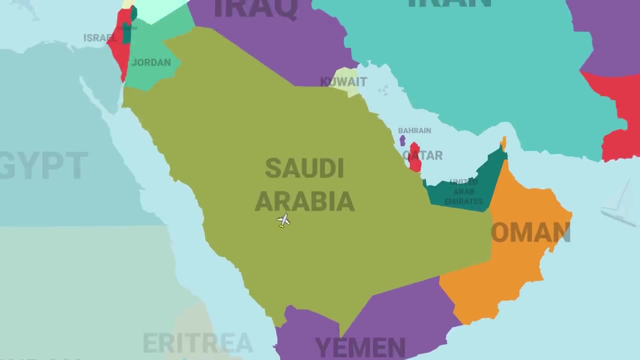 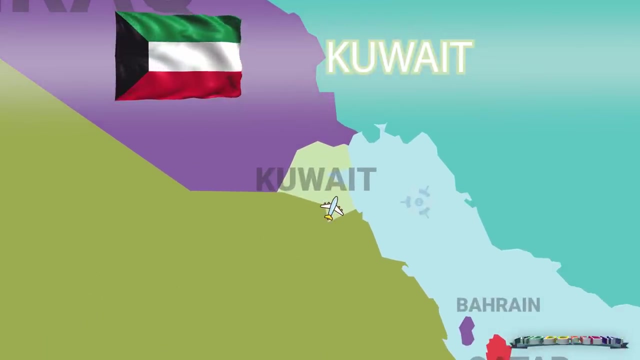 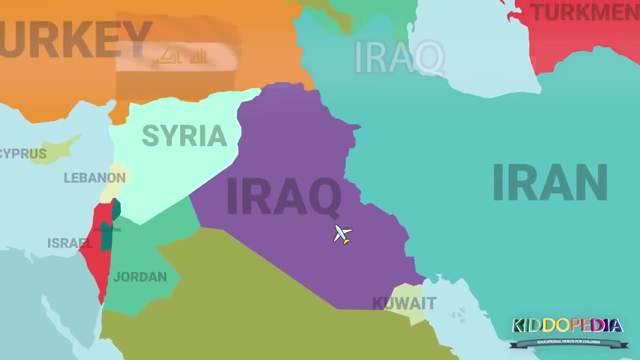 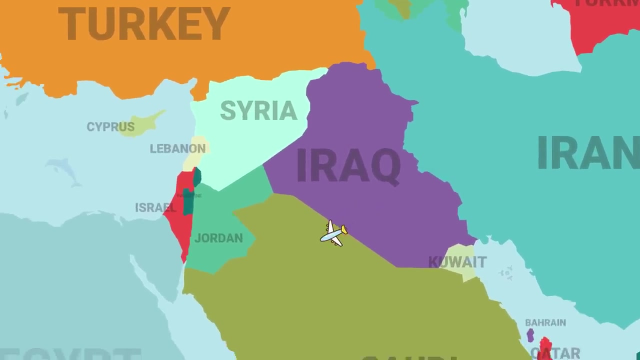 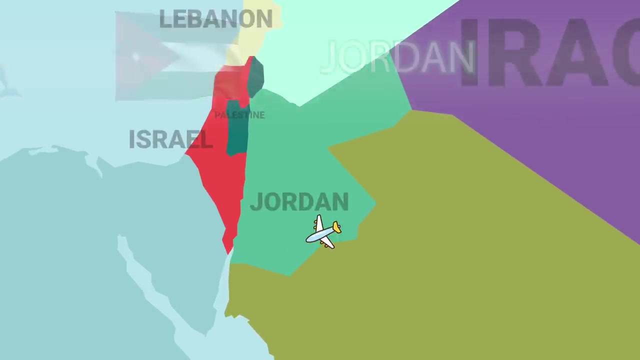 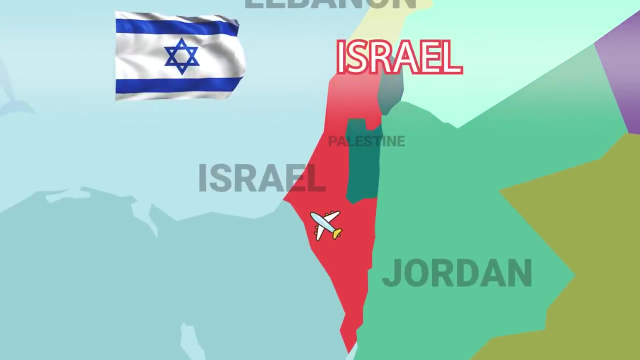 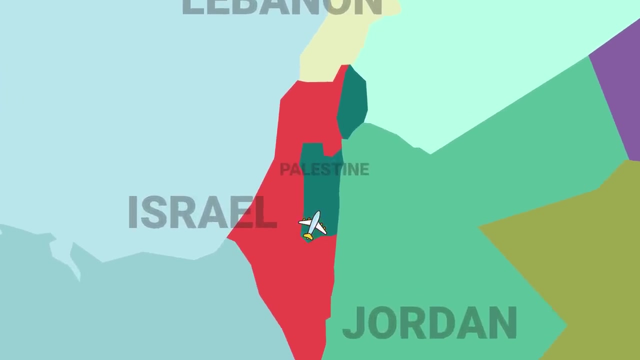 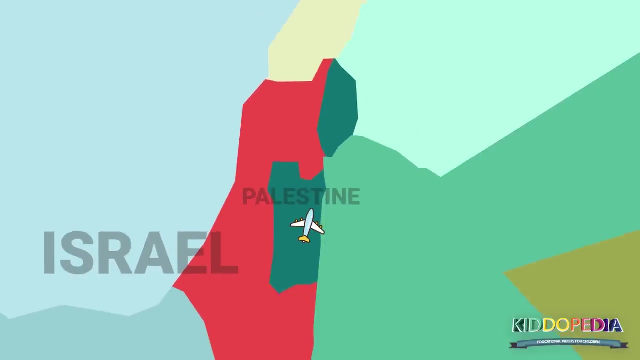 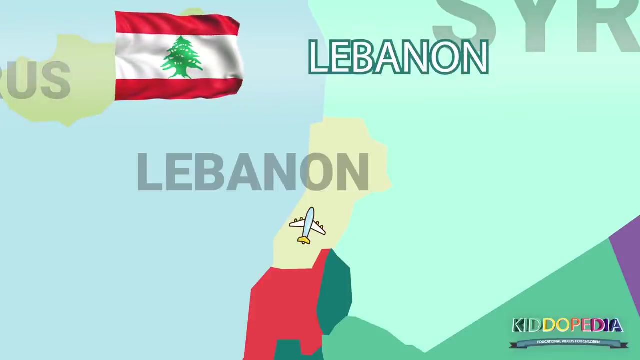 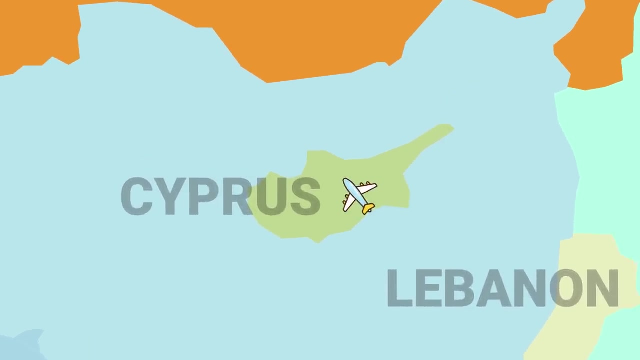 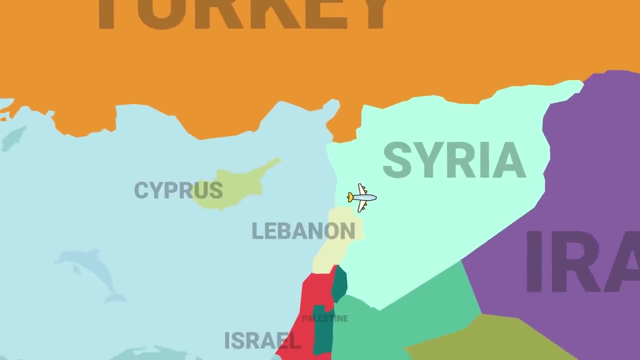 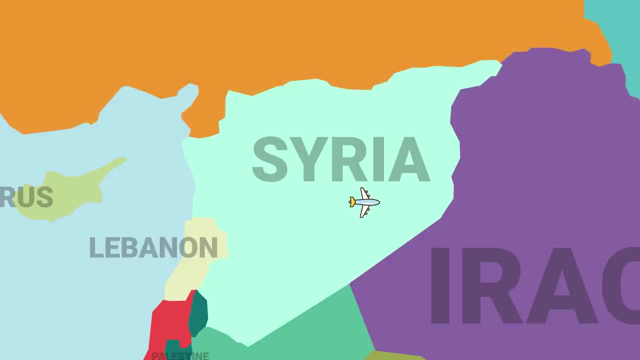 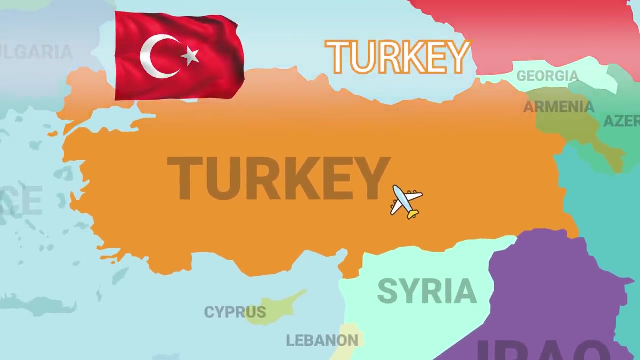 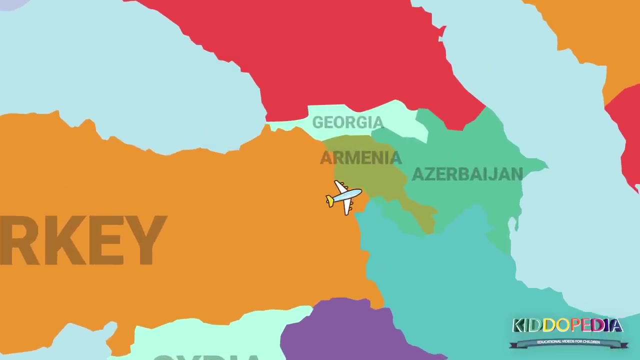 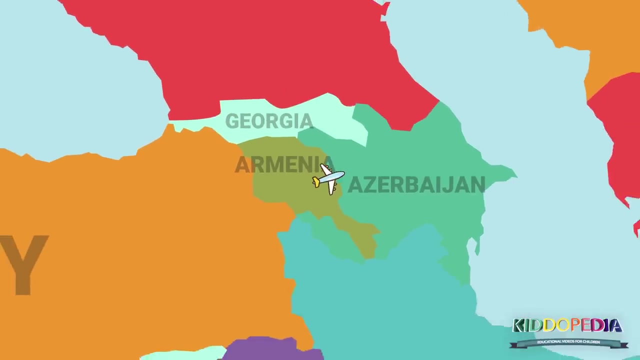 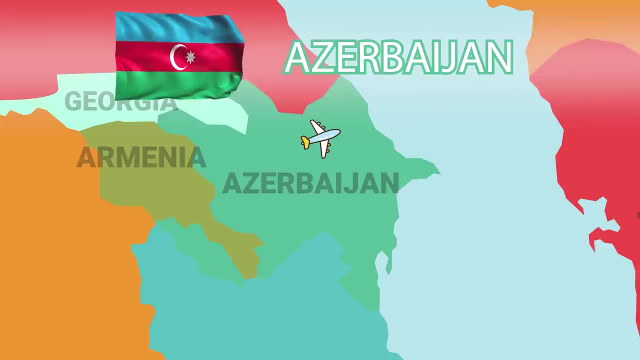 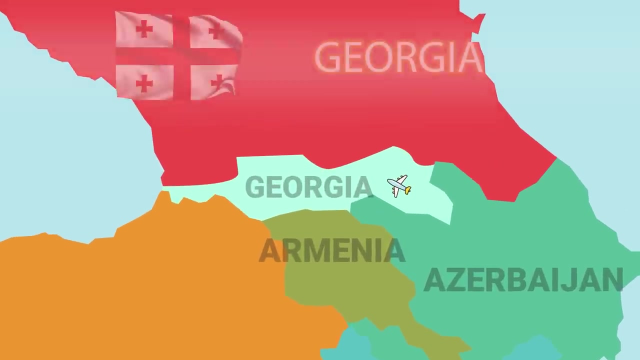 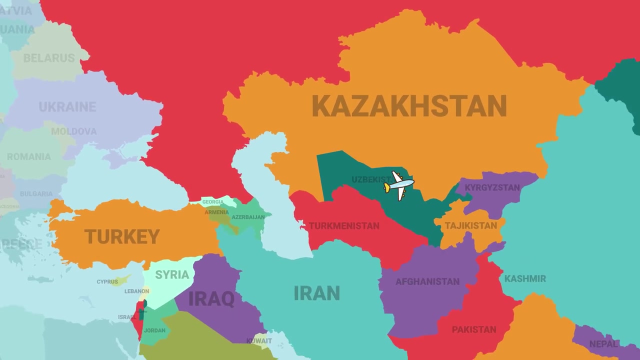 Turkmenistan, Turkey, Iran, Iran, Afghanistan, Pakistan, Pakistan, Pakistan, Yemen, Yemen, Yemen. Yemen. Yemen. Yemen. Yemen. Oman Oman Oman Oman Oman, United Arab Emirates. United Arab Emirates. United Arab Emirates, Qatar, Bahrain, Saudi Arabia, Kuwait, Iraq, Jordan Israel, Palestine, Lebanon, Cyprus, Syria, Turkey, Armenia, Azerbaijan, Georgia. Thank you for watching this video on Kidopedia.